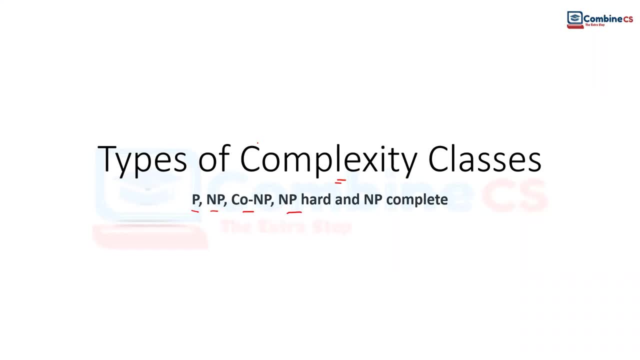 NP-hard and NP-complete problem. Now this topic is again very important for the GATE examination as well as UGCnet examination as well, as you can get the lots of questions in the set examination, and the recent year patterns of the questions that are asked in the examination are very important. 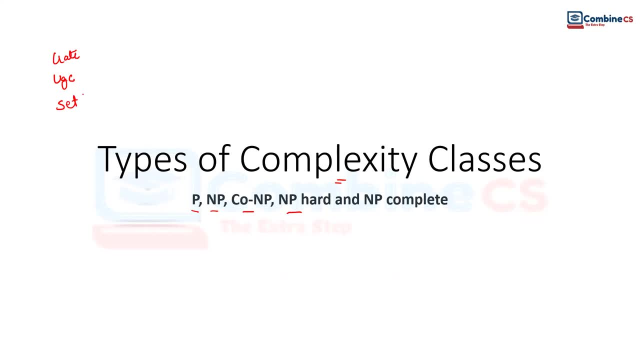 because they also want to know when we are writing an algorithm. So, when we are writing an algorithm, how our algorithm is dependent on the criteria. what are the criterias on which we are going to test an algorithm? So, when we are testing an algorithm, there are two important 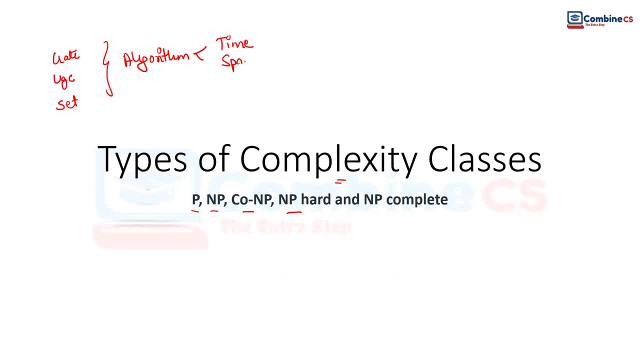 criteria in terms of time, Time and space complexity. And, yes, there are lots of algorithms which have different times and space complexity, So that is already covered In this video. basically, we are going to cover all the complexity classes And this topic is again very important for the data. 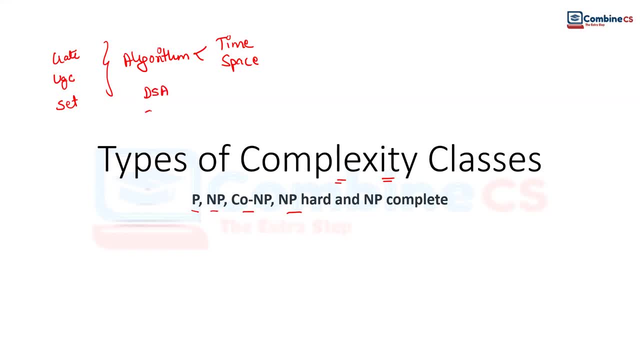 structure and algorithm, as well as the concept, has been used in the theory of computation, And if you talk about the UGCnet examination, we can expect two questions from this topic, and in the GATE examination, we can expect one question from this topic. 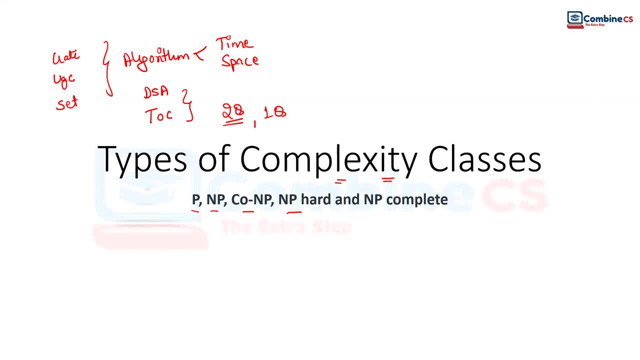 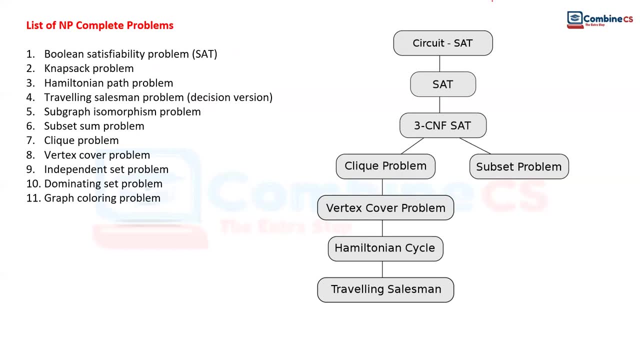 So let's get started. So let us quickly begin our beautiful session and please don't forget to subscribe our channel for all the notification and for all the videos. Now, in the recent year of examination- if you will see net examination- they are simply asking you: what are the NFSAT problem vortex. 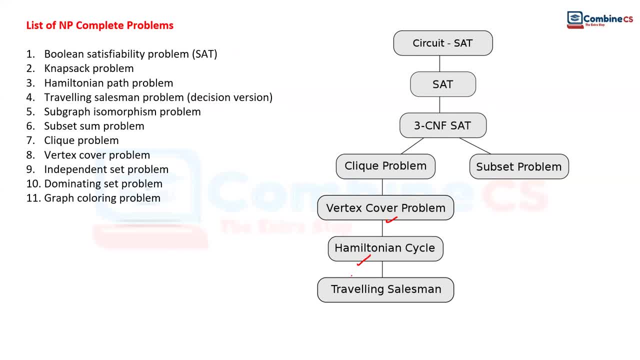 cover problem: Hamiltonian circle: trading sense mind problem. So they belong to which type of complexity classes? So what you have to do is you have to remember this chart. This is the chart, This is the list of complexity classes. So what you have to do is you have to remember and you have to do the following: under the list of complexity classes, you have to do the list of NFSAT problems and you have to do the list of NFSC problem. So what you have to do is you have to remember this chart. So one of the most important point is that 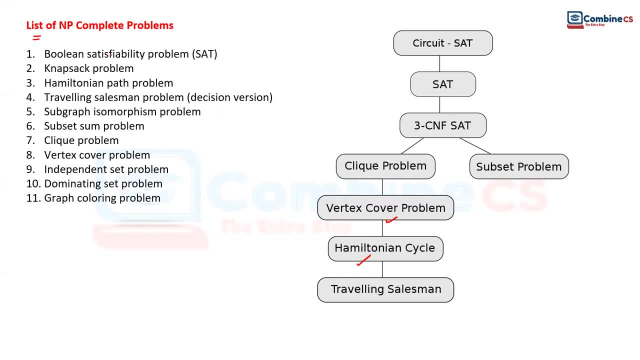 you should know that what are the different types of problems which comes under NPC problem In the short form of this. sometimes you have NPC written in the questions So you can find that in the coming videos that what is NPC. And in the same video I am going to cover 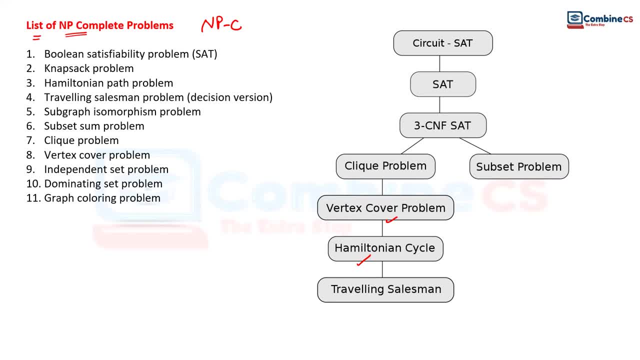 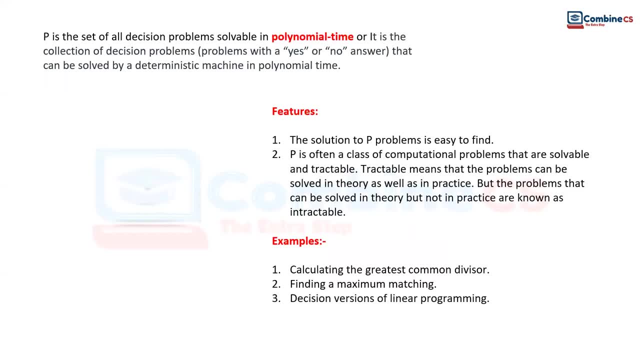 this point. So first of all, you must make this list Now quickly. let us see what are these problems? The first class of family of complexity problem. we are going to cover this. So, if you'll remember this chart, we have the following under the list of NPC problems: 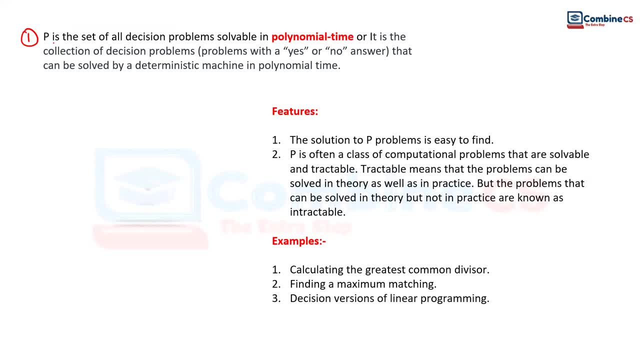 class of family of complexity problem is the P problem. So P is the set of all decision problems solvable in polynomial time. What does P represent? P represents this type of decision problems which you can solve in polynomial time. So that is why it is represented by. 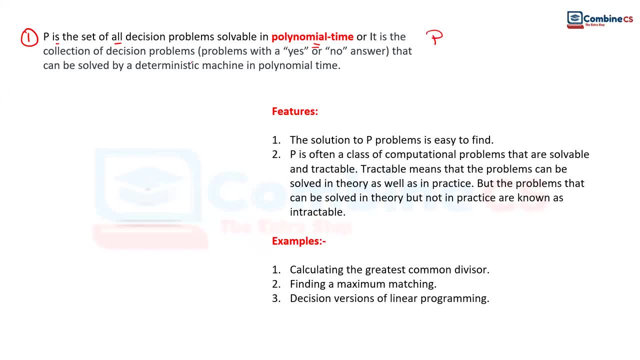 normal P, Or it is the collection of decision problems that can be solved by the deterministic machine in the polynomial time Now here. that is why I told you that if we talk about the P problem, then in the algorithm there are such problems which you can solve in polynomial. 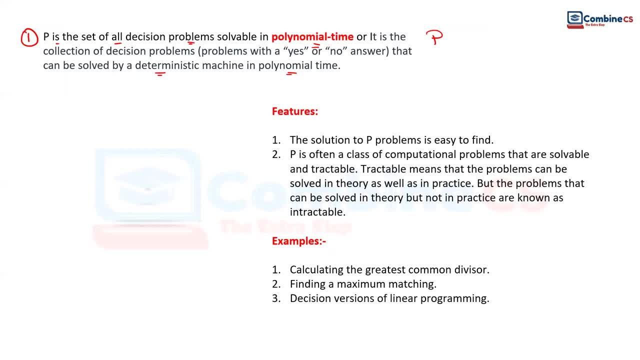 time. That is P problem. And if we talk about the theory of computation, there are lots of machines like deterministic machine, there is a Turing machine, there is a linear bounded automata. So we should also know which type of problem, which machine will pass. And yes, 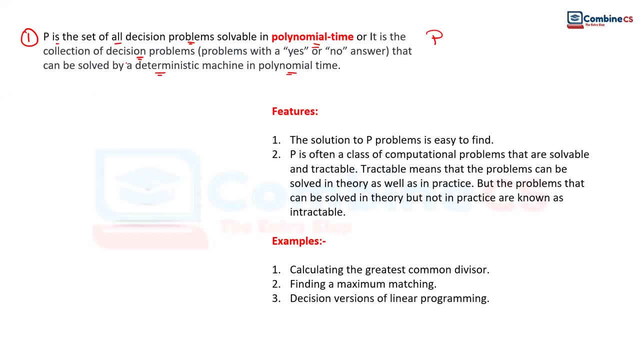 decision problem. if we solve this type of problem, we will get a solution. So that is a problem Can be answered in the form of yes and no. So what does P represent? Polynomial time. You have to remember this. How will you ask the question in the exam? So the question: 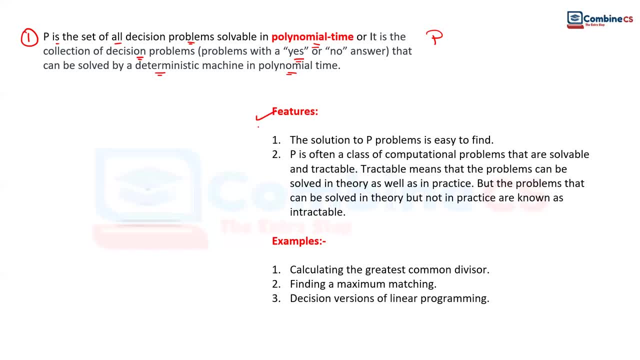 is asked on its features, that which of the given statement is correct or incorrect. The solution to P problem is easy to find Now because the problem can be solved. so that is why it is easy to find. P is often a class of computational problems that are solvable. 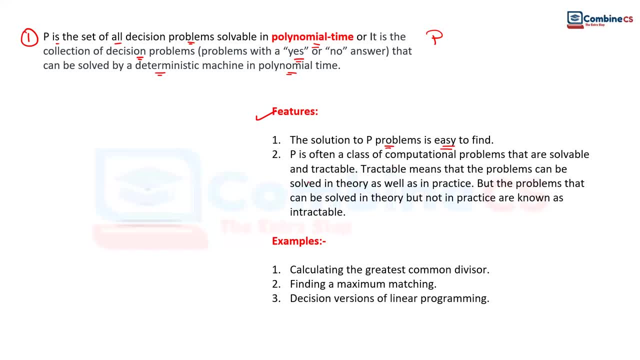 and tractable. Now, once this question has also been asked in UGC net, When we can solve a problem, we can say a polynomial problem is solvable and tractable. If you are solving any P problem, either you are getting the answer in the form of yes or no. then we can. 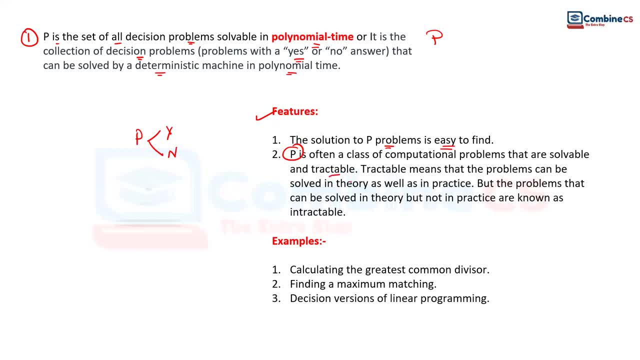 say it is a solvable problem. Now who will? we call tractable? Tractable means the problems can be solved in theory as well in the practice. But the problem that can be solved in theory but not in the practice are known as intractable. So this too has been asked in the examination. 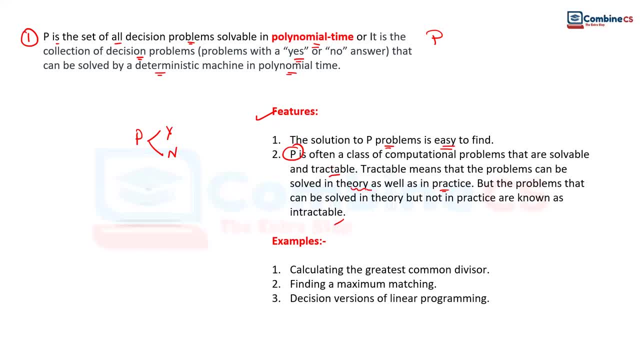 once that such a problem, whose theory as well as practical you are solving, can be solved both ways, This is known as tractable. So all these points should be learned. Now. what are some of the examples that comes under this category is calculating the GCD finding. 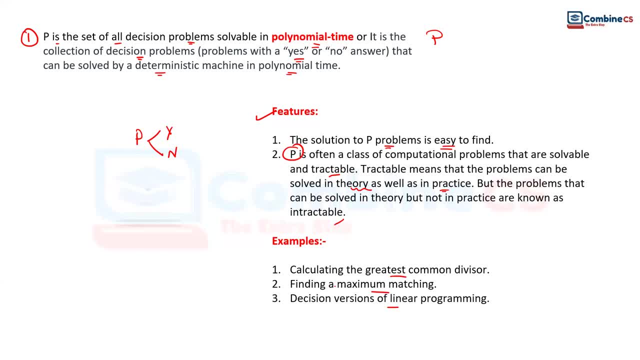 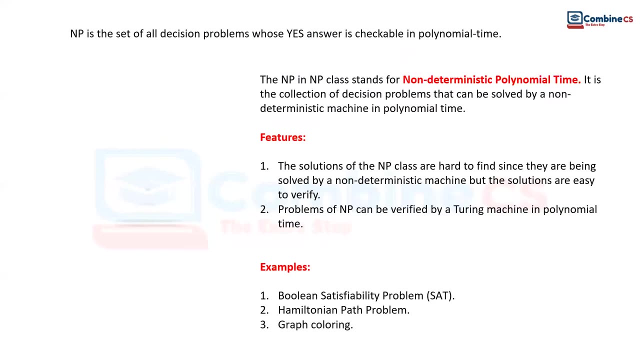 a maximum matching and decision versions of the linear programming. You have to remember some of these examples because it is directly seen in GATE examination and in NET examination. They will give you a list of problems and you have to identify which problem belongs to which category. Let's go to the next problem. This is the problem. Next is the problem which. 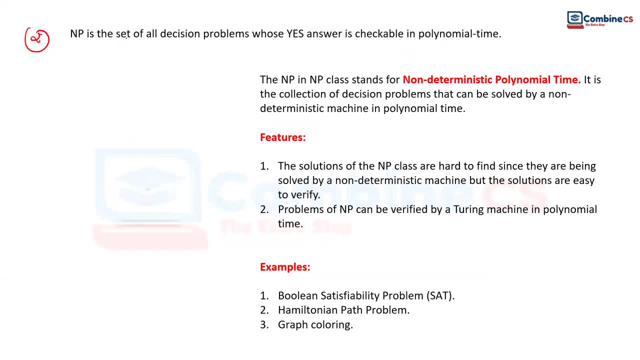 NP. second is the NP. So NP represents the non-deterministic polynomial time. You should also know its full form. and if you have not read this topic in the examination, then also it is such an easy topic. Why? Because the name itself says non-deterministic polynomial time. 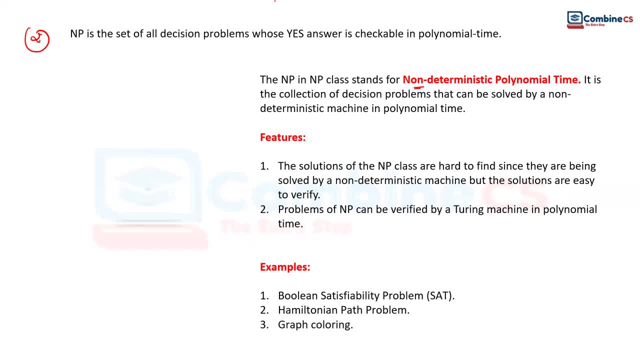 If you are solving a problem but its polynomial time is not determined, it can take too long to execute or to run that program. So that means that problem comes under the category of NP problem. So NP is a set of all decision problems whose yes answer is takeable in polynomial time. 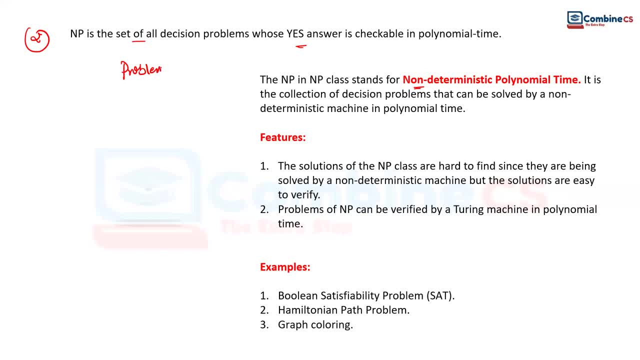 It means that if you are able to solve the problem, then it means that it is solved. It means that the polynomial time is being solved, But if it is not solved, then how much non-deterministic time will be solved that we cannot find. 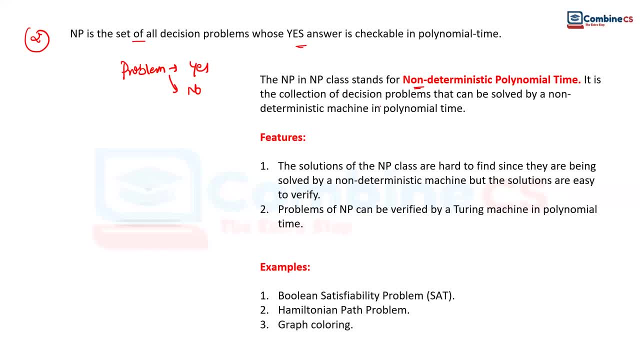 So that is why it is non-deterministic polynomial time. It is the collection of decision problem that can be solved by non-deterministic machine in the polynomial time. So the same definition is written here. And what are the features? The solution of the NP class are hard to find since they are being solved by non-deterministic machine. 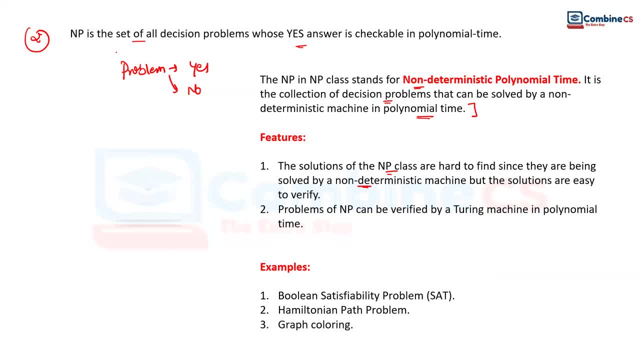 but the solutions are easy to verify. If the problem is solved, it means that you can easily verify it, And if the problem is not solved for any reason, it means that you will have a little difficulty in solving it. here Problems of NP can be verified. 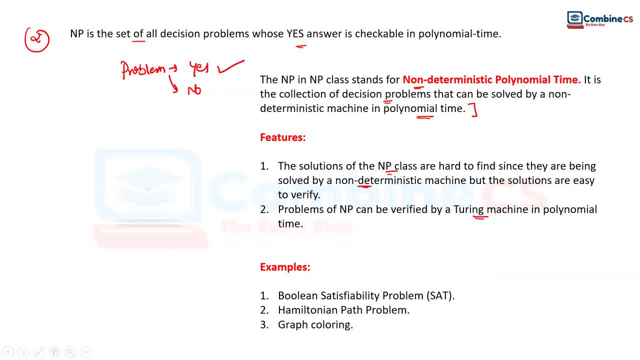 NP can be verified by the Turing machine. So remember what you have to do here. In the previous polynomial we saw that you will solve it through the deterministic machine And you will verify the NP problem through the Turing machine. So you have to remember these small points. 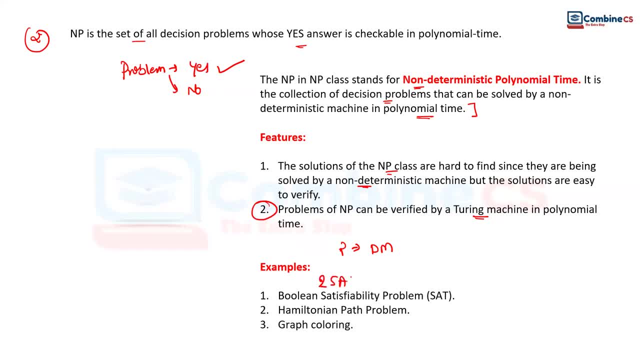 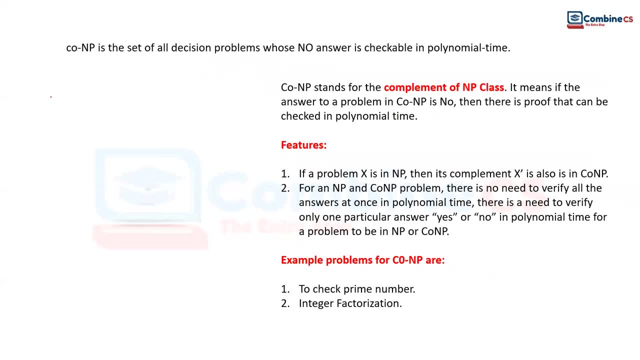 Bowling satisfiable problem, which is also called two set problem, Hamiltonian part problem and graph coloring problem are some of the examples of NP complexity class. The third important category is CONP, That is the set of all decision problems, So no answer is takeable in polynomial time. 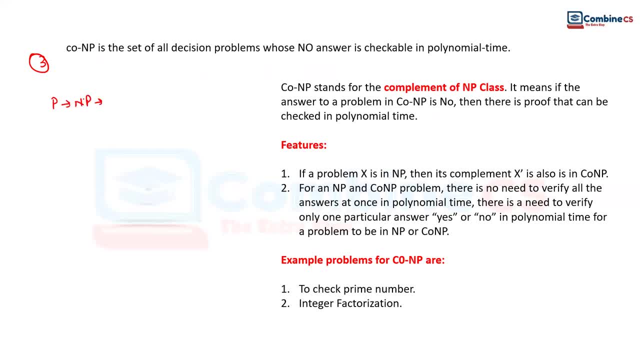 So you have to understand that if we read P first and then NP, then our complexity is increasing. Next, in this we were getting the answer of both YES and NO. Here we were getting only the answer of YES. And what will we get in the CONP? 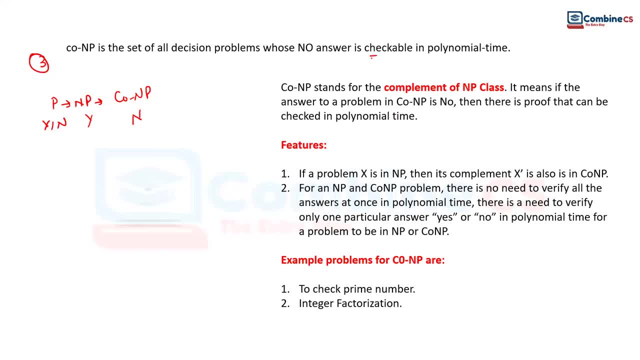 In this we will also get the answer of NO. No answer is takeable. So in this way, you can make short notes. CONP stands for complement of NP class. Now, this name is very important. What does CONP represent? 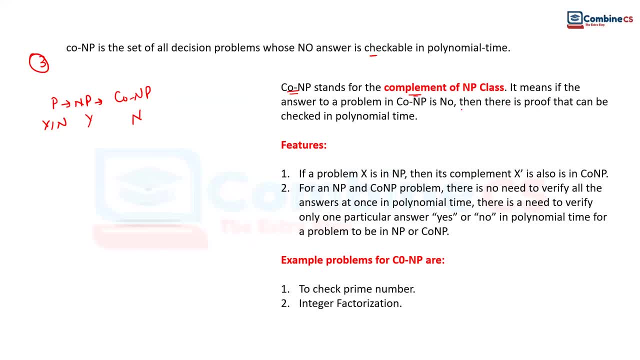 CONP stands for complement of NP class. It means if the answer to the problem in PONP is NO, then there is a proof that can be checked in polynomial time If you are not able to solve any problem due to any reason. 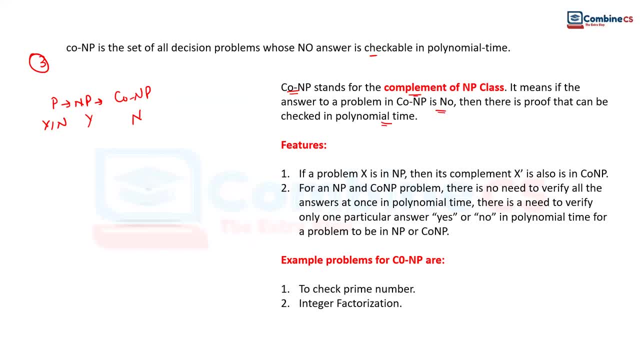 still we can give the proof that why we are not able to solve the problem. So, even if there is no problem being solved- I am repeating again- if we are not able to solve a problem, but still we have proved that we are not able to solve this problem. 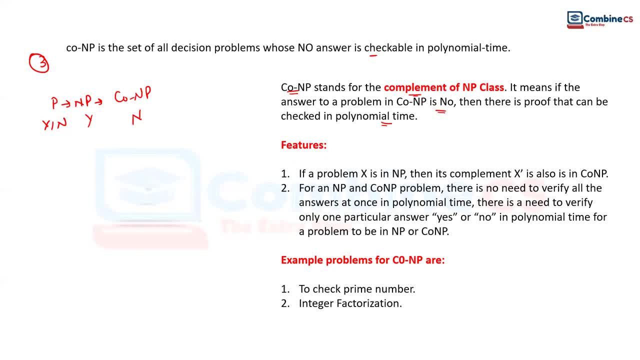 it means we have come to some certain conclusion, So we can say that it will be a complement of NP class. So what are the features? If a problem X is in NP, then its complement X bar is also in the PONP. 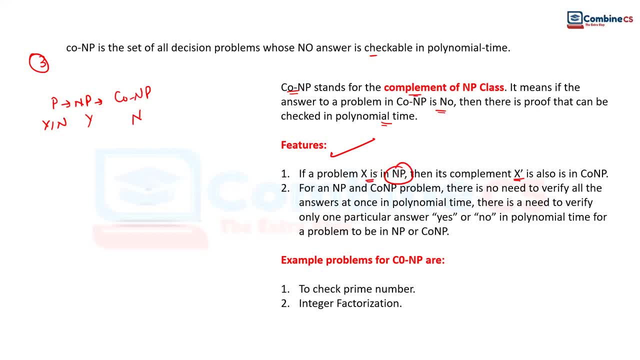 So you have to remember some of these theories that if a problem is in X in NP, then its complement will also be in PONP class For NP and PONP problem. there is no need to verify all the answers at once in the polynomial time. 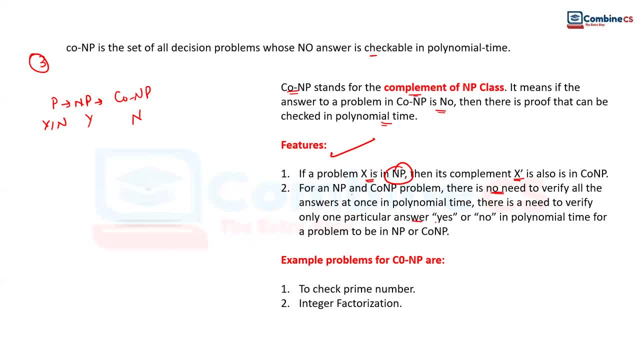 There it is a need to verify only one particular answer- YES or NO- in polynomial time- For a problem to be NP or PONP. So here it is said that you can verify any one problem. That is fine, Okay. Examples to check the prime number: integer factorization. 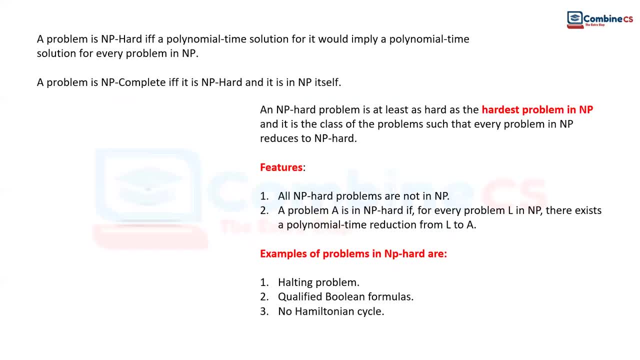 So you have to remember what the examples will say in its categories. Moving to the next, is NP-hard. What Now, while a problem is said to be NP-hard, if the polynomial time solution for it would imply a polynomial time solution for every problem in NP? 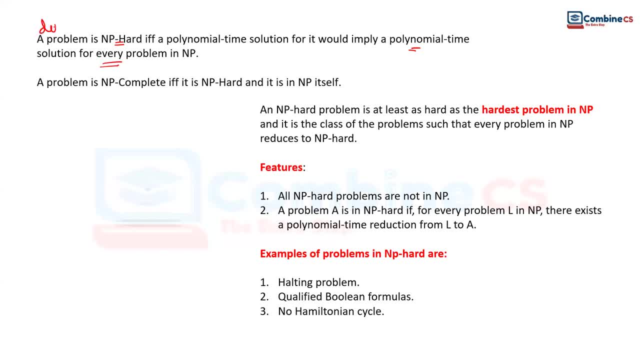 Now, if you look at the net examination, then on this definition, only many times your question has been asked. So what is the important point Here? it is IF. This means IF and only IF, And here they will give at most instead of EVERY. 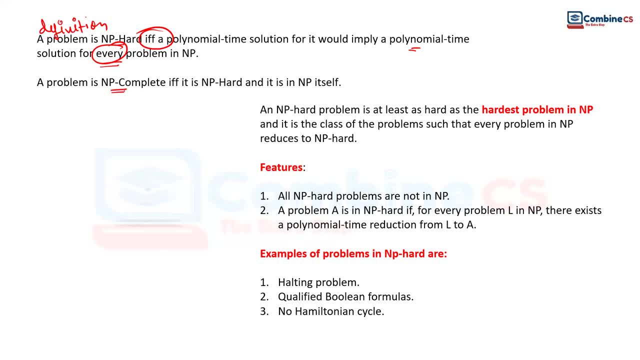 So you should learn all these lines. A problem is in NP-complete, if it is NP-hard and if it is NP itself. It may be that when you watch this video it will be difficult for you to remember some of the problems, But do not leave the video. 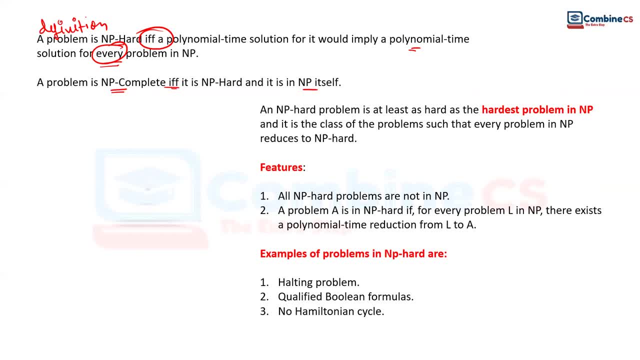 because now I will represent it with a diagram immediately. I will tell you a trick so that if you watch this one video, then you will be able to solve every question of the complexity class. So stay tuned till the end of this video. Now, an NP-hard problem is at least as hard as hardest problem. 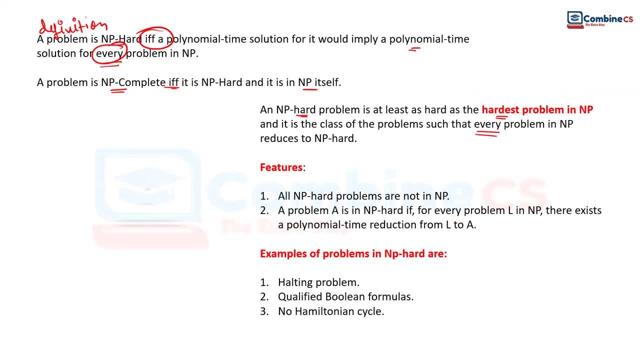 See, it is NP-hard. It is clear from the name itself that all the problems should be reduced in NP-hard. All NP-hard problems are not in NP. Now what is all this? I will explain you first, Then we will move to these points. 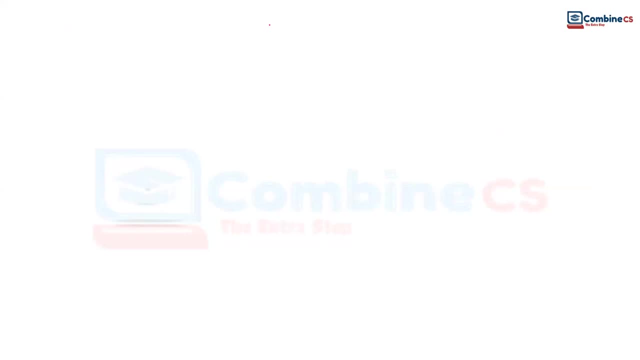 Okay, See. So to understand this problem, I have also made a video in theory of computation, So let me explain you here. If a problem is given. if a problem is given, then it can have only two solutions. Either you will be able to solve that problem. 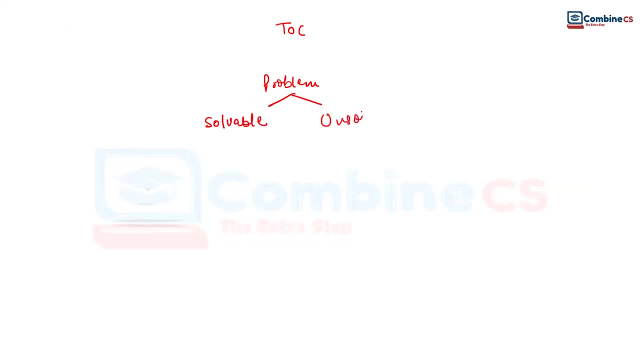 we are able to solve that problem, or else we are not able to solve that problem. There will be no 50-50 situation. Either you will get the solution, otherwise you will not get the solution. Now, if we have solved any problem. 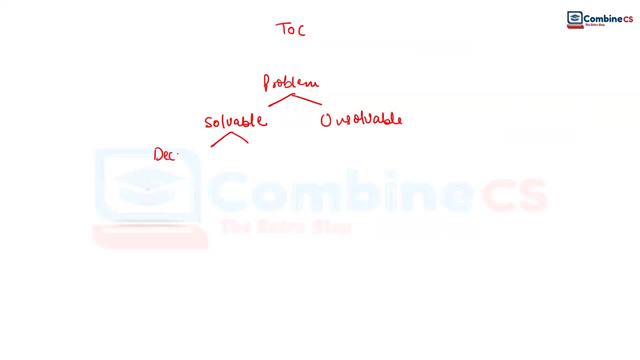 then it has two important cases: Either we can decide it- that means it will be decidable- or it will be undecidable. Now this topic is again a high-weighted topic in the theory of computation, So many learners have doubts about it. 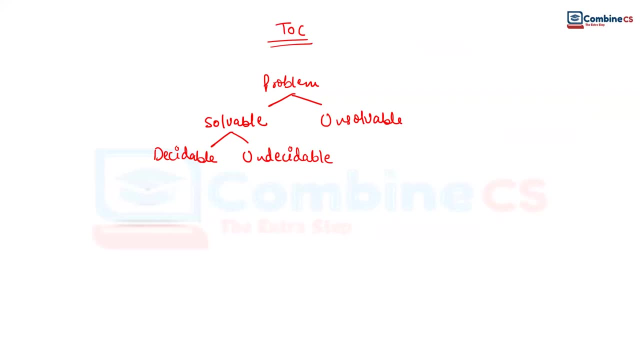 That is why I am covering this topic here too, Because if you understand the concept, then you will be able to solve both the questions. The meaning of decidable is that, to solve this problem, either we will be able to solve it in polynomial type. 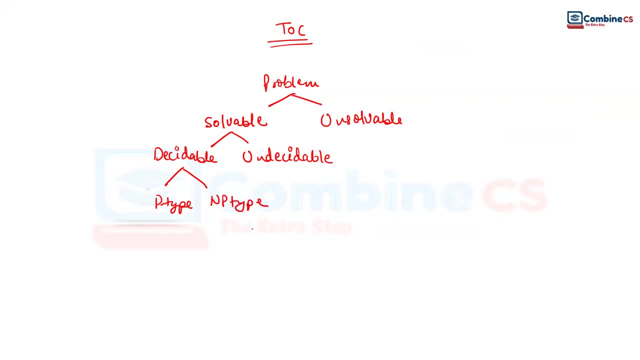 or we will be able to solve it in non-polynomial type. Okay, Now we have learned what is polynomial type and what is non-polynomial type. What is it So, this problem which we are able to solve in polynomial type? 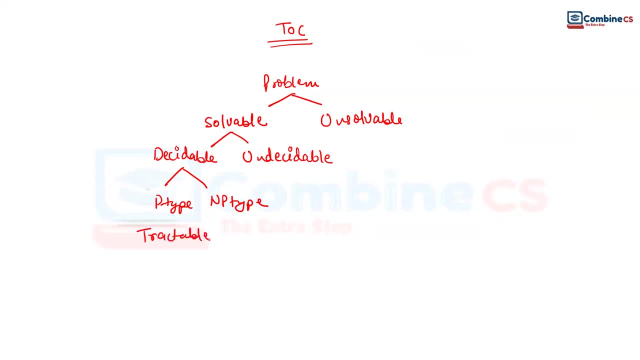 should I say that we will call this problem tractable. Just now we have seen that its theory as well as practical. We can solve this problem in both ways. Similarly, we will call it intractable. Why? Because here, when we get the answer in no 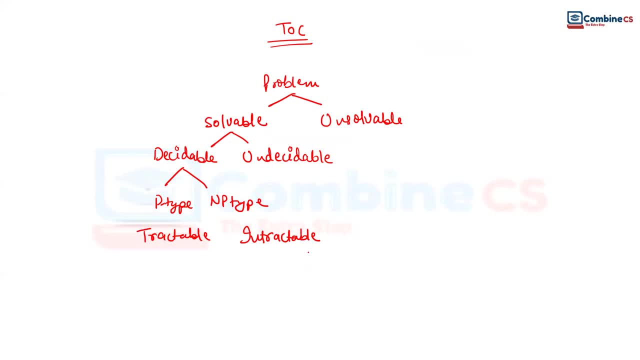 then we cannot identify how much time period we have solved it And the problem that is undecidable. should I write this Because all these problems are very complex And in net examination and gate examination also, questions are not asked from it. 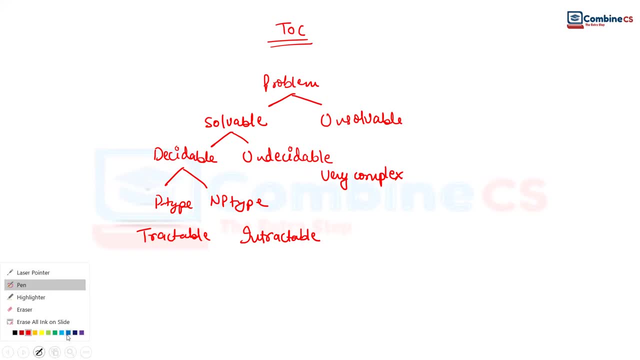 Basically the questions that are asked to you. they are asked from the decidable property, And what is not decidable it means that it is an undecidable problem. So you have to remember this chart. Okay, You can also understand the meaning of decidable. 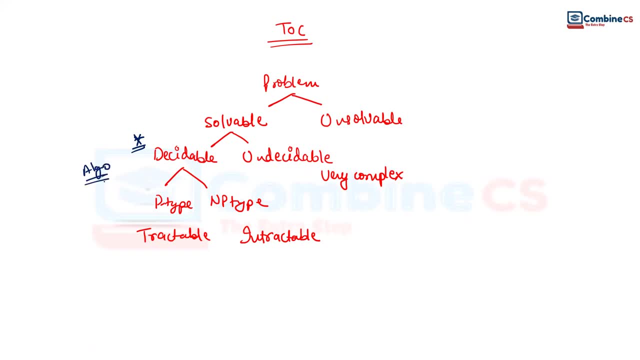 that we have an algorithm to solve any problem. That is why we are telling that this is a decidable problem. Okay, This is the way to represent it. Suppose this is our universe of discourse. There will be some problems here, which we will solve in polynomial time. 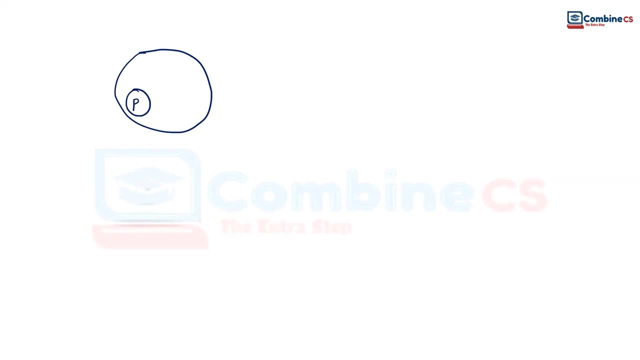 So in a large part we have solved some problems from the universe. And then how will all the problems be solved? There will be NP problems. If we are able to solve something from all the problems, then we are not able to solve anything. 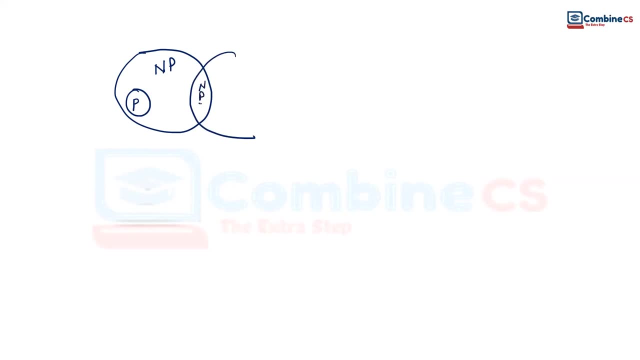 After that we will take some in the intersection And this section will be your NPC, That is NP complete And this will be your NP half. So this diagram is very, very, very important. I am telling you again, There are many types of problems in any universe. 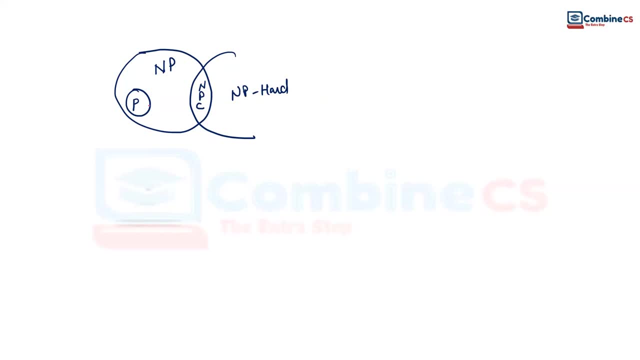 Some problems will be solved, Some problems will not be solved. So some problems which will be solved, you will call it polynomial P type. So that is why this problem will come in which category? It will come in the easy category, And the rest I make a sigma star here. 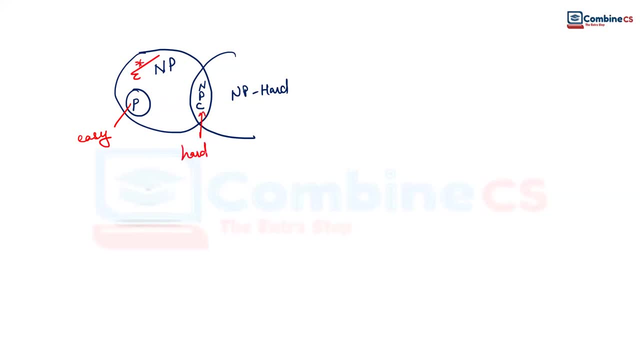 All the problems will come here. NPC, you have a heart problem here which we will not be able to solve, And NP heart is such a problem which you will never be able to solve. They are unbounded. There can be many unbounded problems here. 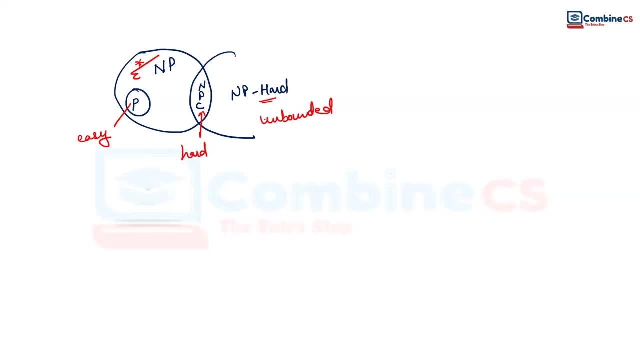 And this is a full form: NPC, complete or NP, heart. Okay, Now some questions will ask you in this way. For example, if I write P1 in this way, what does it mean? It means that we can reduce P1 in this P2.. 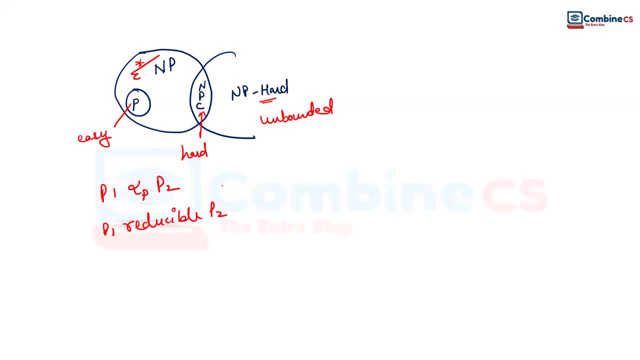 You have to remember these terms- which is written like this, And you will see this question in the examination many times. So it means reducible. Okay Now, moving to the next point. I hope you have cleared this diagram. Now I will go to the slides at the back. 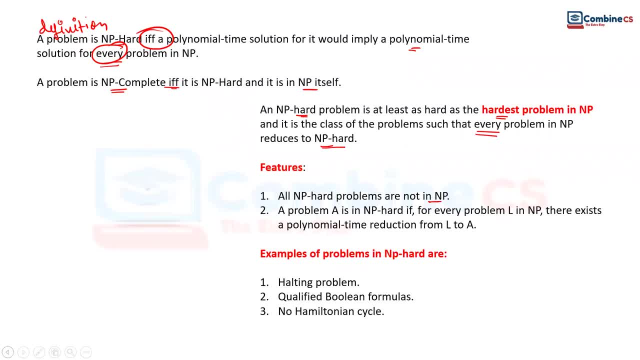 so that you can understand that statement. So this was the thing. So a problem is in NP complete if it is NP heart and it is NP itself. So now we have seen that this is a problem: P NP and here your NP is C. 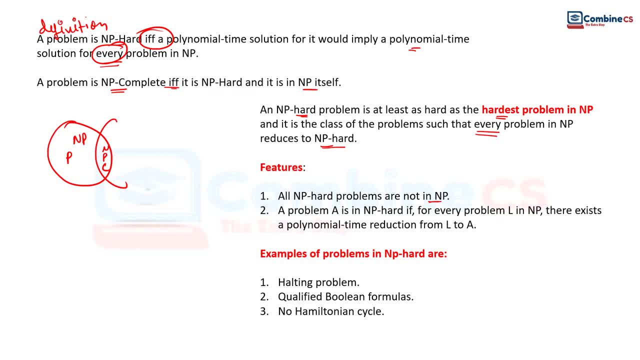 So if you ever get this type of question, what will you do In the examination? the rough sheet you get, you will make this problem there. You will make this diagram. Then you are going to solve that problem. So that problem will be solved easily. 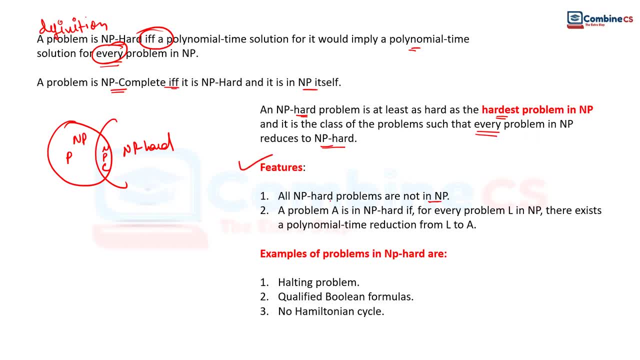 and you will get the answers Okay. Its features are also: yes, All NP heart problems are not in NP. Now this statement will be verified from here. If there is any NP heart here, then how can we say that all NP heart problems? 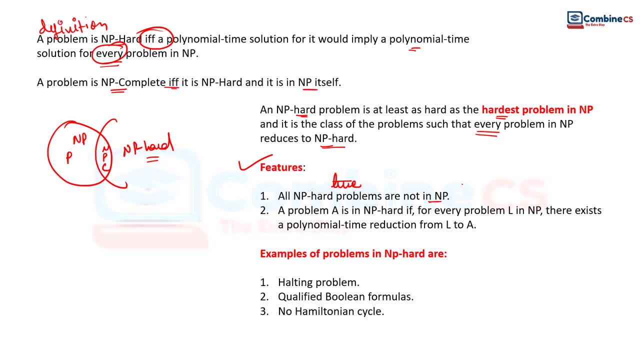 will be NP here. So this statement is true And this statement again is the previous year question of UGCNet. They have asked you in the true and false. Now problem A is in NP heart. Let's go. I will make a problem here. 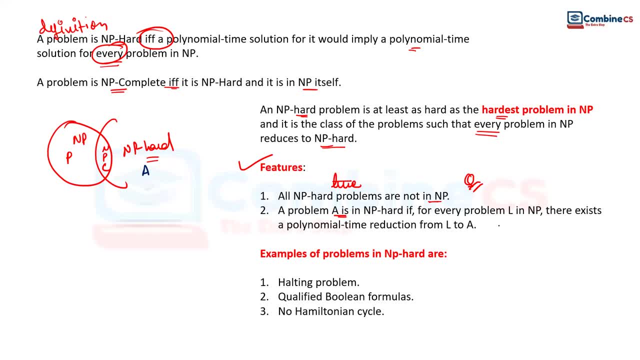 This is a problem. Here is A Okay For every problem: L in it. What does L represent? Language, Any language. Let's suppose I take this L language. So this is the statement of theory of computation. Language, Language can be anything. 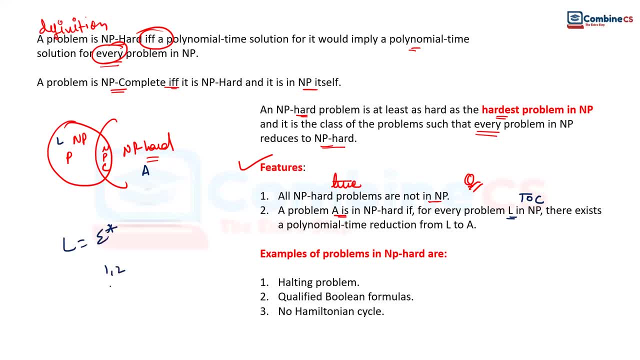 You represent it with sigma star. It can be 1,, 2,, 3,, 4.. It can be ABCD, It can be any symbol. This is how we define language For every problem. L, L. in NP, there exists a polynomial time reduction. 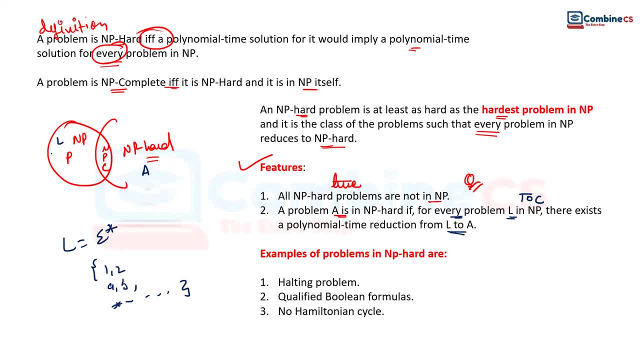 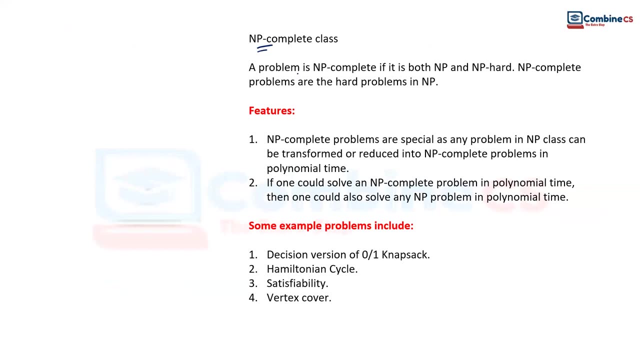 to language to A. So if any language depends here, then obviously some languages will be like this, So you can reduce it. Why? Because somehow these are the easy problems as compared to NP heart problem. These are some examples given Now. this is the last family, NP complete class. 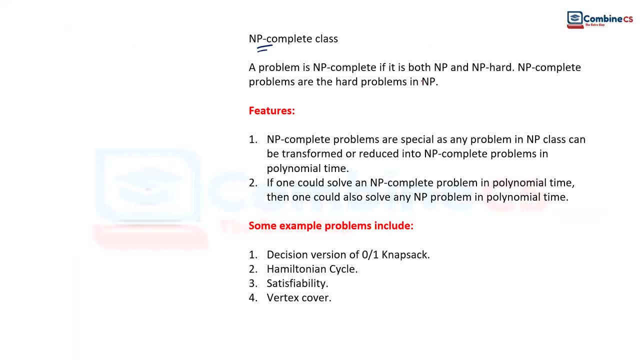 A problem is in NP complete if it is both NP heart NP and NP heart. Okay, What did we see? There was an intersection here. Okay, And these are the heart problems in NP. NP complete problems are as special as any problem in NP class can be transformed. 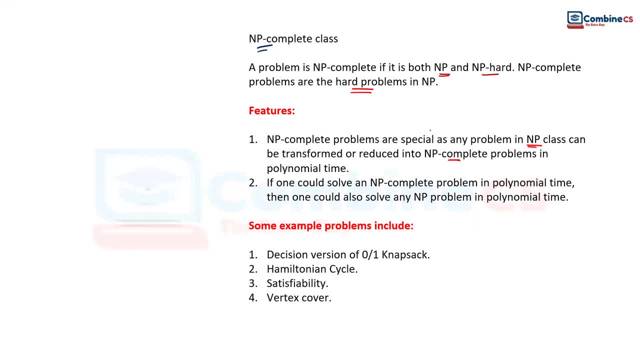 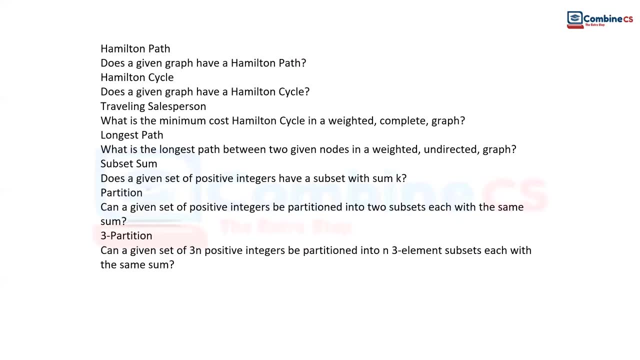 or reduced into NP: complete problems in polynomial time. This same thing has been written here in turn, So don't go into so much difficulty. What you have to do is you have to remember this chart. What kind of problems are there Solvable? 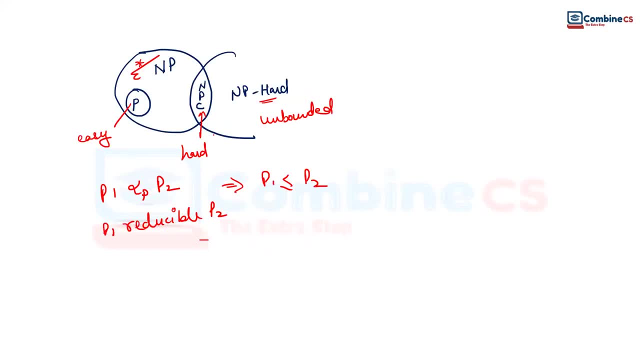 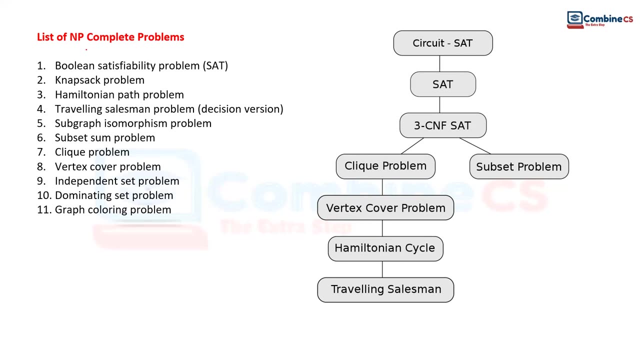 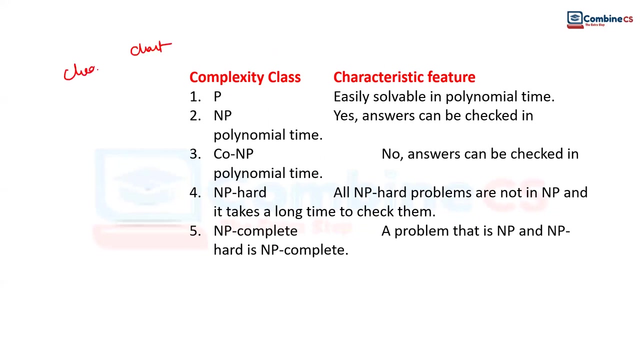 unsolvable, decidable, undecidable. Okay, And remember this diagram. After this, from the exam perspective, you will remember this chart that all these problems fall under the category of NP. complete And remember this chart. This chart is called a cheat note. 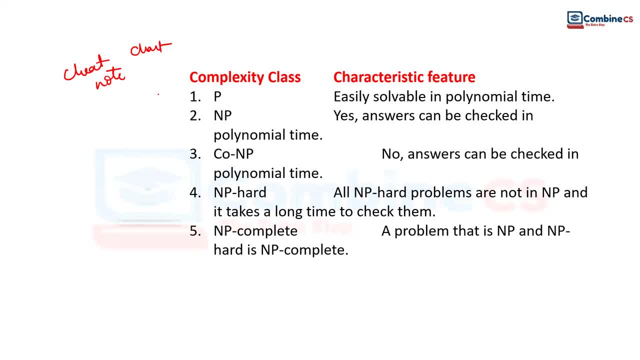 Don't take a cheat note in the examination. It is just to remind you: P represents easily solvable in polynomial time, NP represents yes Answers can be checked in polynomial time, The algorithm of which you can give only yes answer. we will be able to check it in polynomial time. 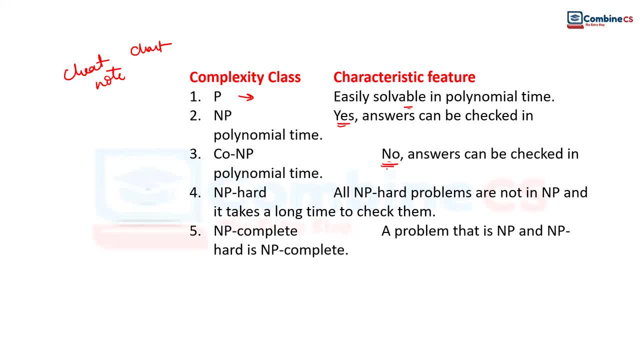 Co-NP means complement, In which we are also able to check no answers. NP heart means all NP heart problems are not in NP and it takes a long time to check a problem, A problem that is NP and NP heart is NP complete. 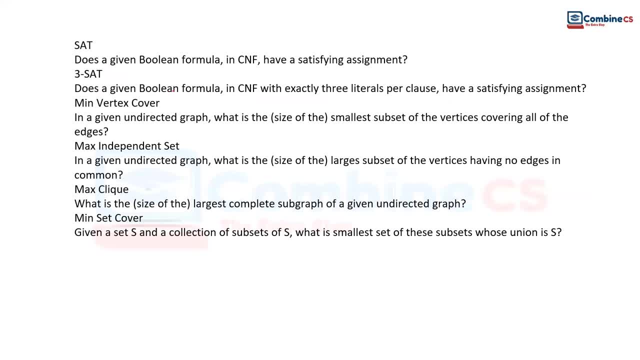 So you have to remember this cheat note. Many times it has been seen in the UGC net that we will simply ask you what is the minimum set cover? What is the max independent set? So that's why I have given a small definition here. 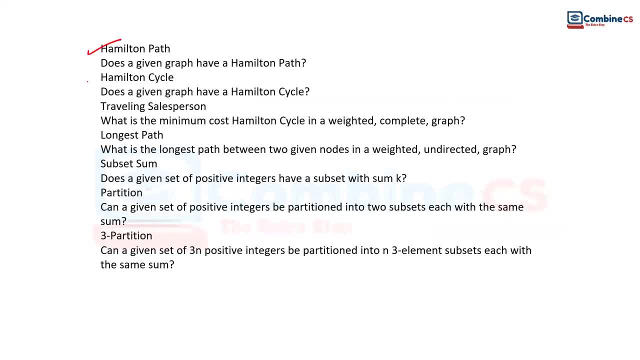 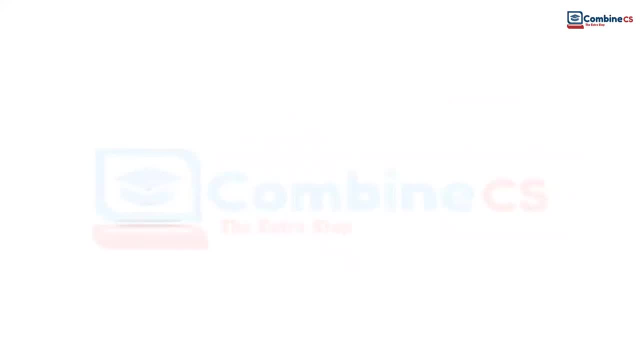 You must check it once. Hamiltonian path cycle. So this all comes under the category of NP complete. Now we have read this, You will also solve some previous year questions of UGC net and gate. on this, Like a simple question is asked. 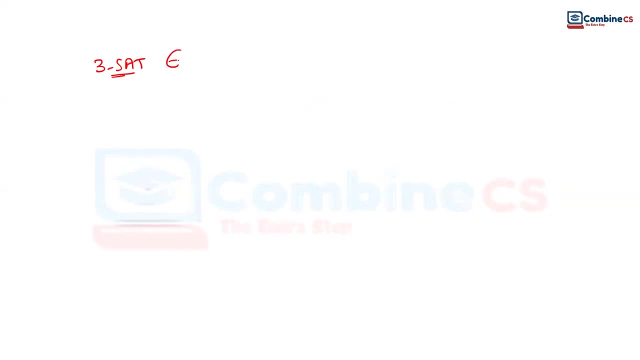 what is the three set problem? Three set problem is it will belong to your NP complete, So you will remember this. After this: the two set problem: this problem comes to you in P problem. So this is directly the previous year question of UGC net and gate. 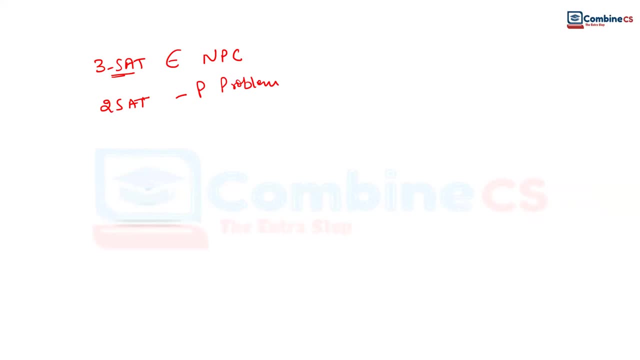 And in UGC net. simply, your question is coming directly from the gate question and there is nothing explanatory in it. If you remember some points then you can easily solve the question. So you have to remember this: that which problem comes in which. 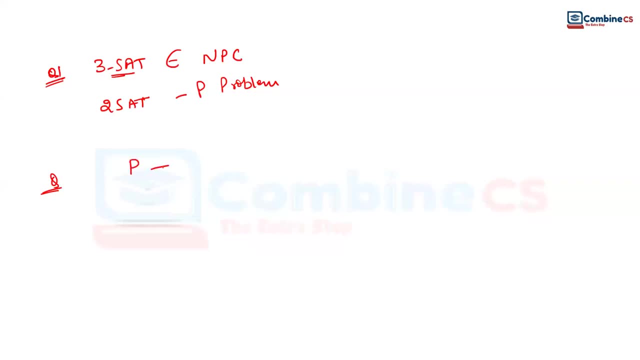 After this, I will ask one question in this way, that this is P, which is given that it is not equal to NP. Here I have told that P is not equal to NP, So what can you get out of this? I will give you an option. 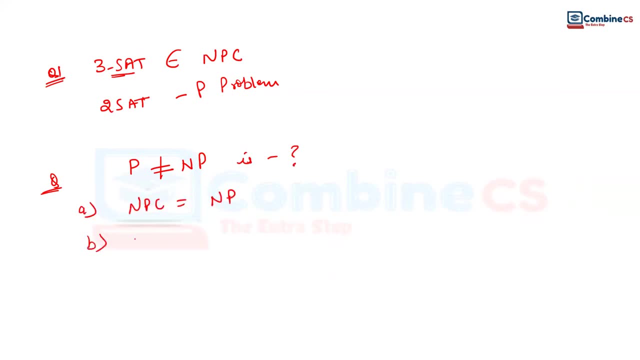 NP is equal to NP. What will this mean? Yeah, NP is intersection. If I take its P, then it will be 5.. Let's ask C question. So this is the question given here. Yes, So this is the question here. 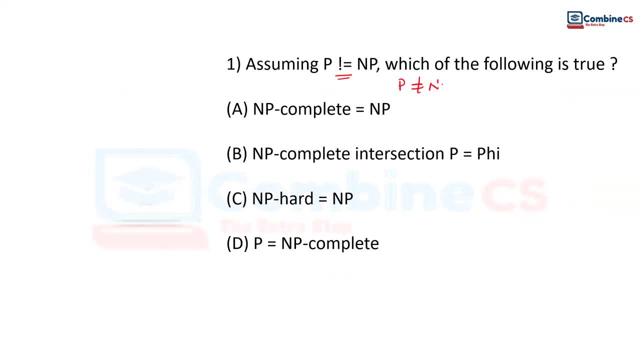 Assuming P is not equal to NP, P is not equal to NP, So which of the following statement is true? So please make this question a diagram, As I make a diagram here. Okay, P is NP here, So this is the wrong diagram. 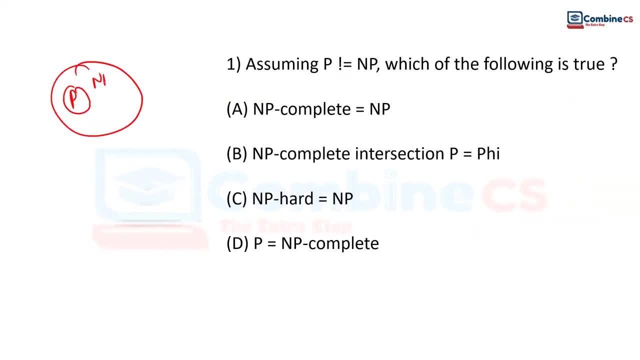 So this is P. Okay, this is NP. Then here I will make NP C And here I will write NP hard. So this is clearly given. here P is not equal to NP. Which of the statement is true? You have to tell. 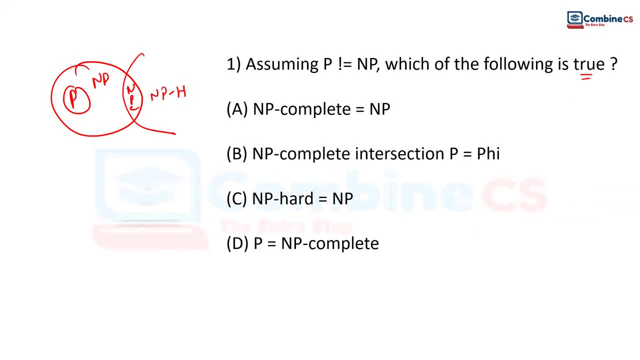 So P is not equal to NP. What will this mean? Okay, so if you see, NP will be equal to NP. No, we just saw this now. NP hard will not be complete with NP. This is also not equivalent to it. 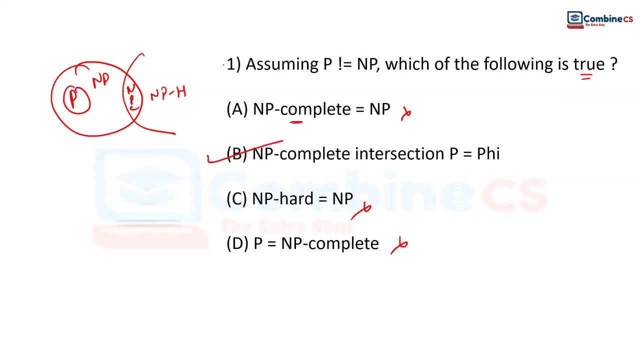 So it means that, after eliminating all three options, this is our answer. So this is the gate previous year question. It is a question of 12 marks, So you can solve it on the basis of this diagram in this way. Let's look at the second question of 2006.. 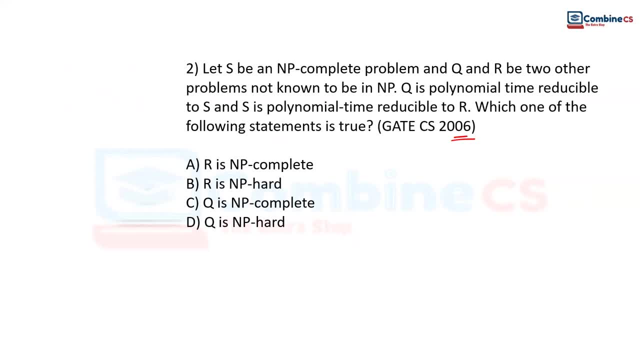 And there are a lot of chances that this question will be asked directly on your UGC network. Let S be an NP complete problem and Q and R be the two other problems not known to be NP. Q is polynomial term reducible to S. 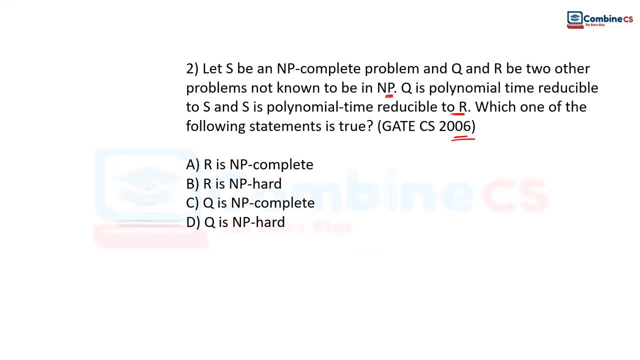 and S is a polynomial term reducible to R. Which of the following statement is true? You have to take P, Q, R as the concept of reducible. You have to make a diagram in this way and you have to put these values here. 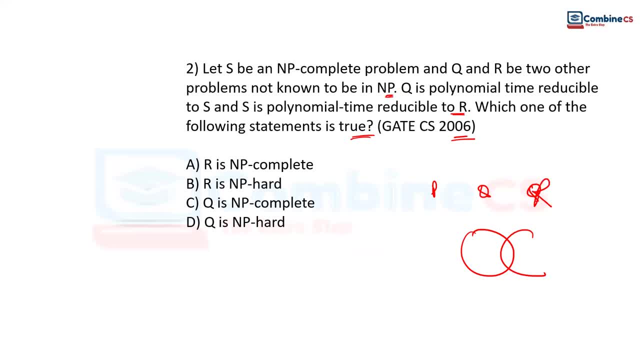 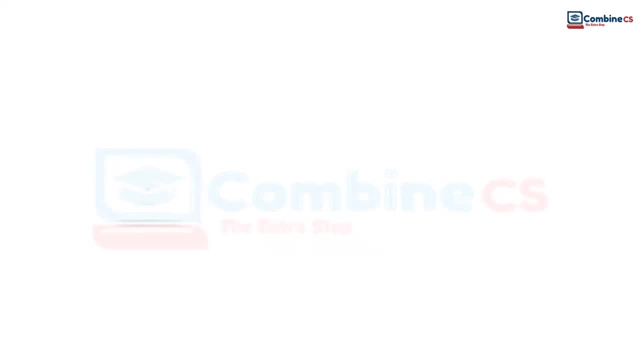 Then you are going to solve this question. Please give the answer to this question in the comment section. Okay, After this, some questions have been seen that there are long questions. But yes, if you know the concept of decidable, then you can solve these questions easily. 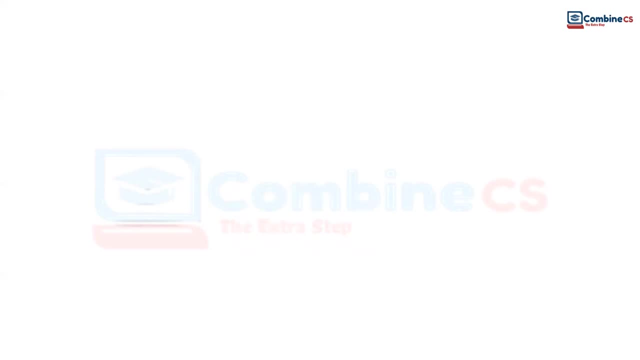 Simply, such questions have also been asked once, Like we will give you there. Suppose there is an algorithm of polynomial time which is computing the largest, which is Q, Okay, And how can you represent this in the diagram? So now you should know here that